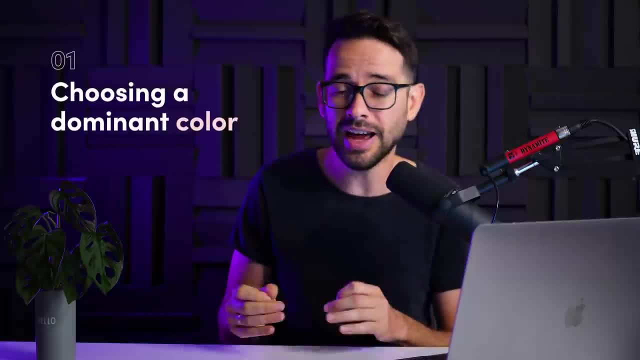 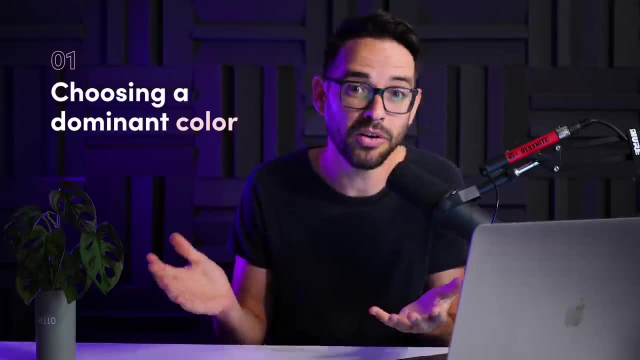 process. Step number one: choosing a dominant color. Now a lot of your clients might come to you and they already have kind of a brand color and that's great because you have step number one figured out right. But if you don't have that step figured out, you need to choose the right. 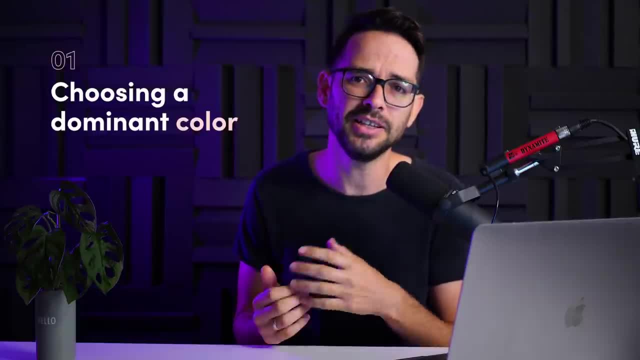 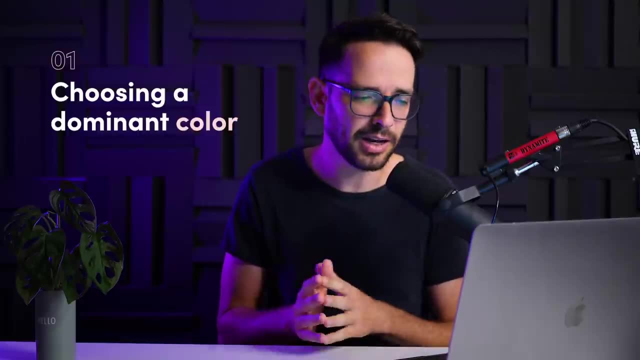 dominant color for your client, And that basically means that you need to understand what is the meaning of every color, right? And so let's take the example of Phlox Academy and the color palette that we've created for it. So we got started using this dominant color, which is a 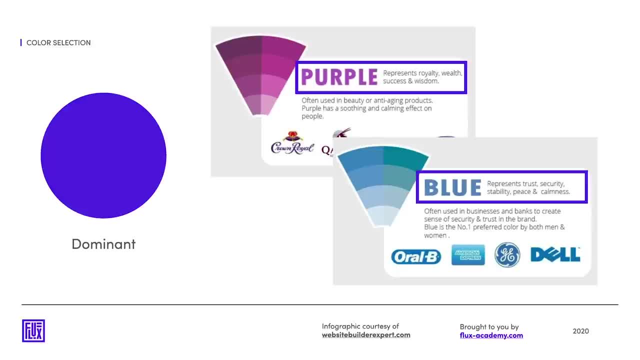 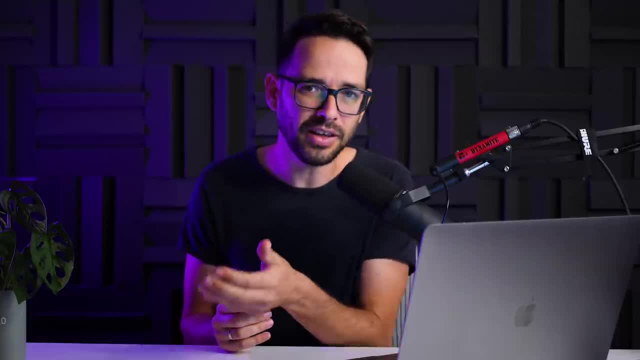 combination, kind of a color between purple and blue. Now we have to understand. what does it mean if we use these colors, and I think that they actually convey the right message for our customers. Now we'll share below a link where you can find the meaning of every color, but in this: 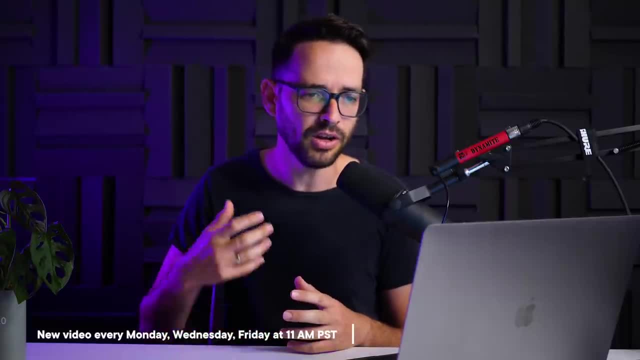 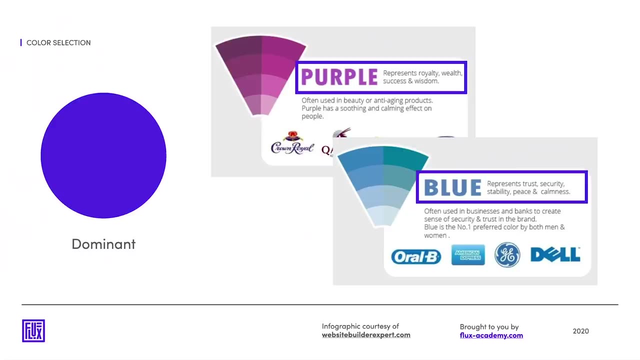 example, we only have a purple color, So the dominant color or the general meaning of purple is usually something like wealth, success and wisdom, which is not bad for a school. And then blue is always represented by trust, security, stability. That's why most of kind of like 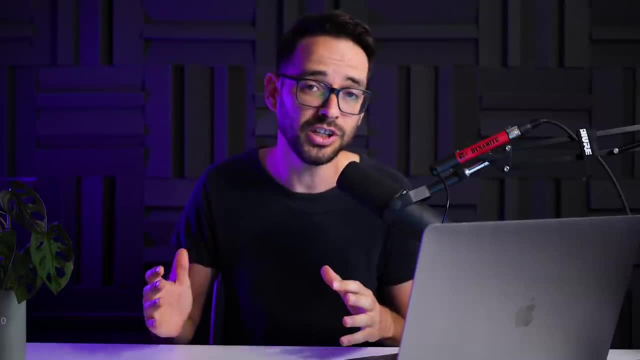 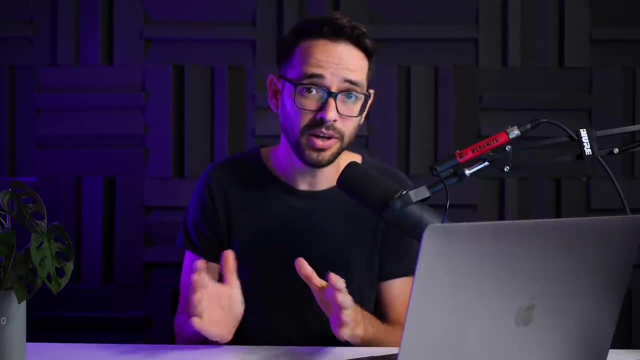 businesses, big businesses use it, So it's very kind of like solid color. So a combination between them is something that is pretty good in terms of meaning for what we want to convey with an online school. So that is the dominant color we got started with. 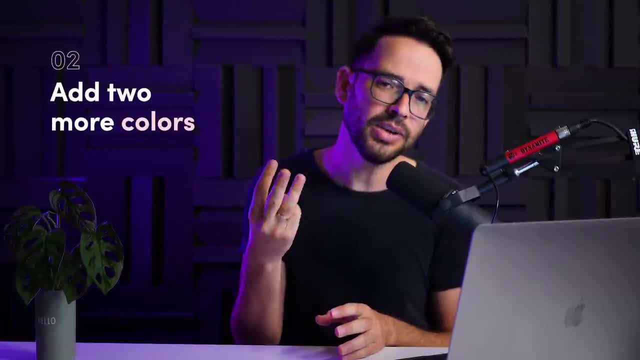 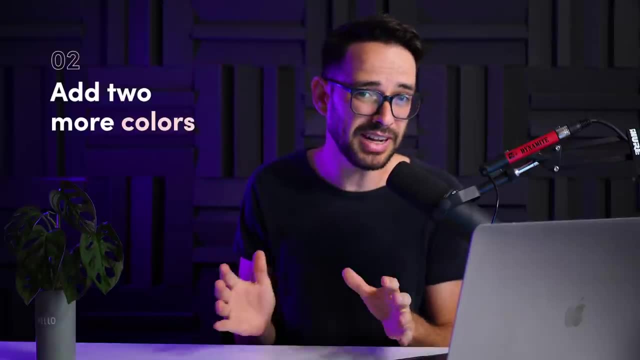 Now the step number two is to add two more colors so that you can have a palette of three colors. Why three colors? We'll get to that when we'll talk about how you're gonna apply those three colors, But the next step is: let's find what other two colors 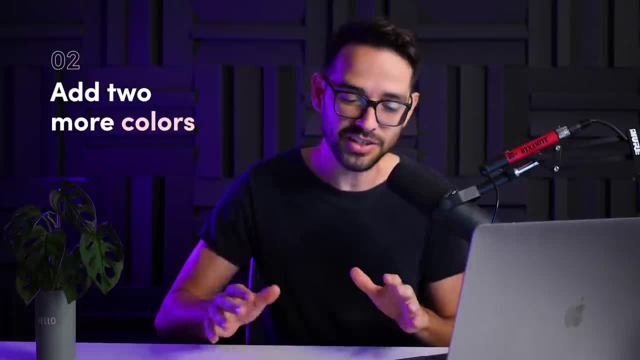 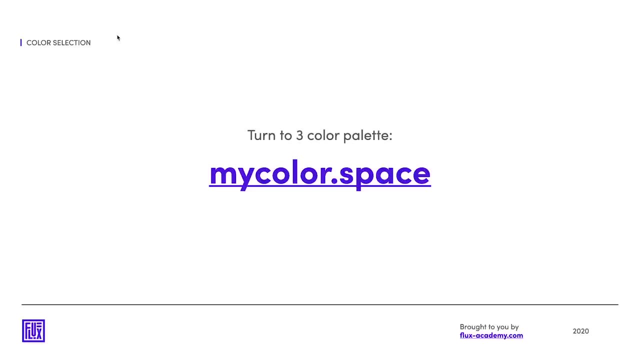 are gonna work well with this dominant color. Now again, because I suck at this, I always try to find tools that are gonna help me kind of brainstorm the ideas. The tool that I wanna share with you right now is called My Color Spaces. 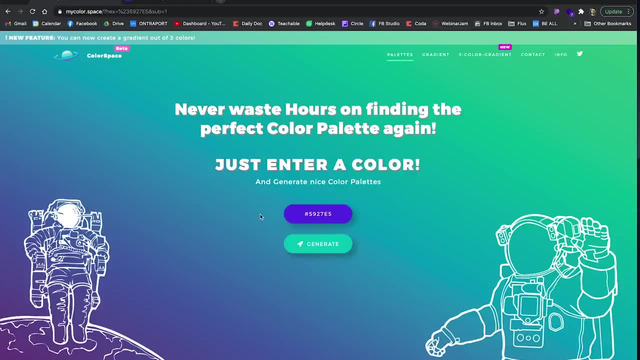 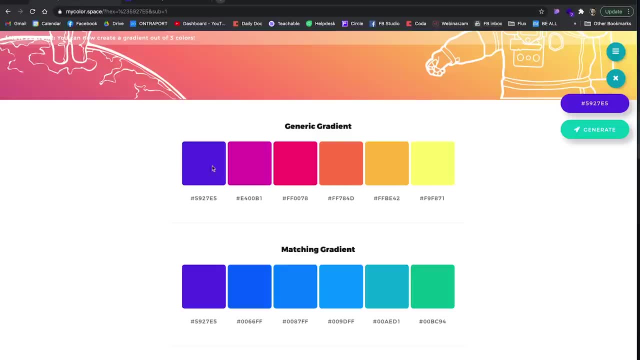 Basically, you just enter a color, So in this case I've added the color that we chose as a dominant. Then we create, generate And basically it creates a bunch, of, a lot of palettes that are just basically working with this dominant color. 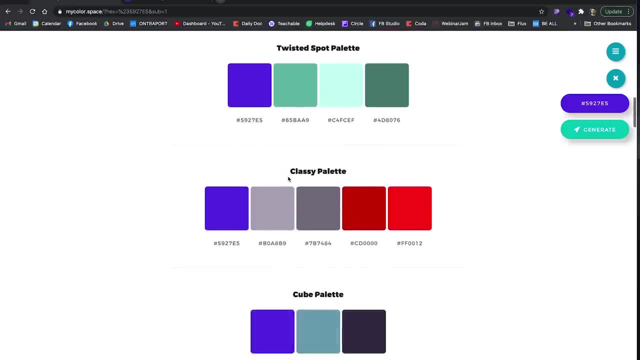 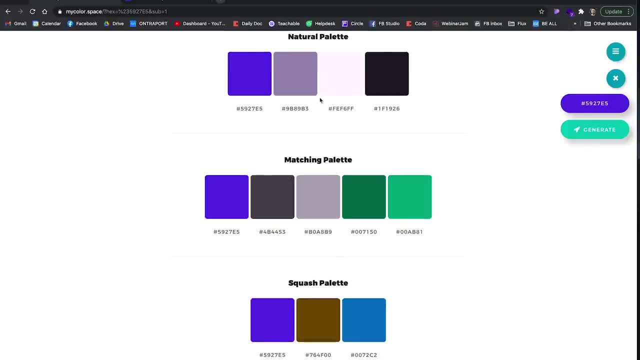 So, as you can see, there's gradient matching color, like a bunch of them, like a lot of them, right, And so this basically serves as, as you can see, they're not all three colors palette And but this basically serves as an inspiration. 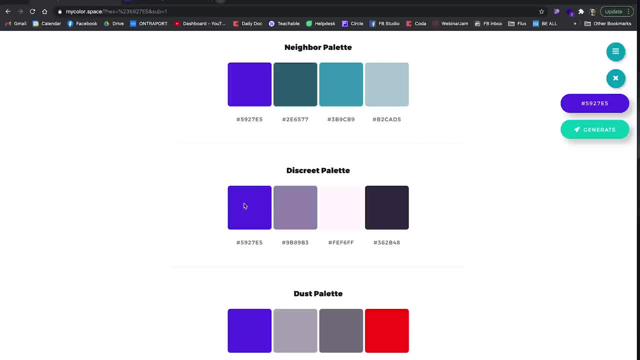 for what can work. So for us we went with something that is not very functional, Far from this right. So we have this purple, we have this kind of a very light pinkish, and then we have this kind of a very dark. 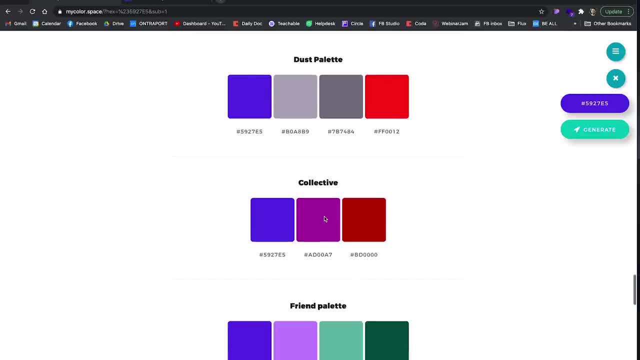 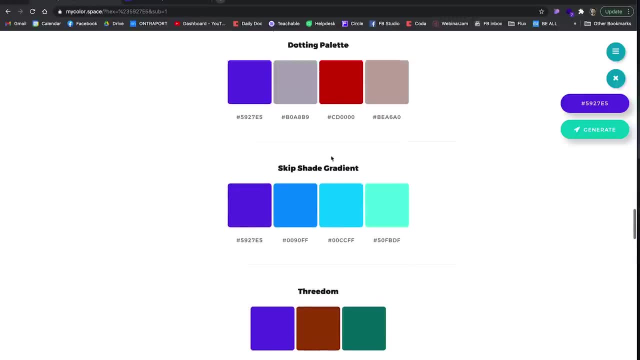 And we chose to simplify this using black. So this website is again very, very helpful to kind of brainstorm what other colors are gonna work well with your dominant color, And you can use this to kind of get the general direction and make your selection based on that. 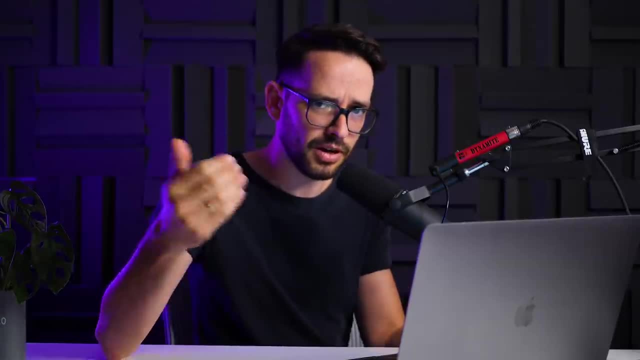 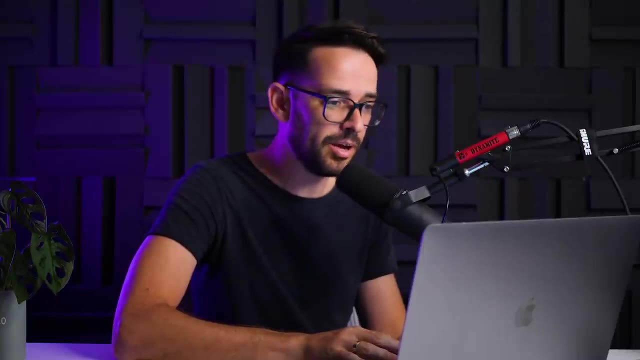 By the way, if you find these types of videos helpful, just like this video, So we can know, and YouTube knows, that this is helpful for you and then we'll keep doing more of these. Anyway, back to the palette. So here's the palette that basically we came up with. 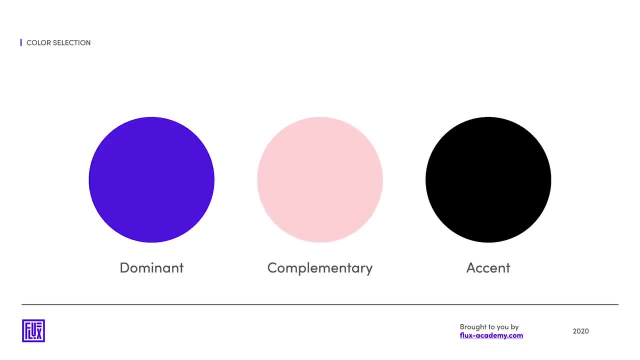 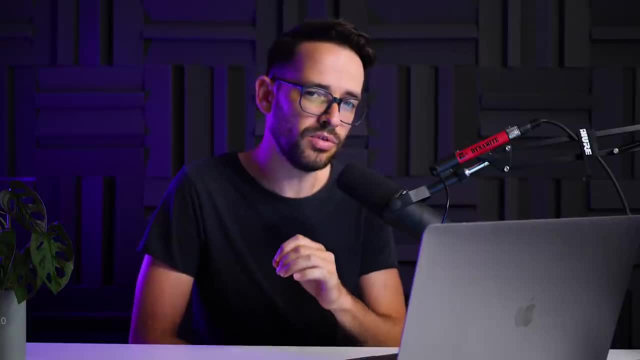 So we chose the purple, we chose a very light pinkish, and then we went with a black as kind of an ascent for it. Now, by the way, I think something that a lot of people don't think about when they think about color: is that black? 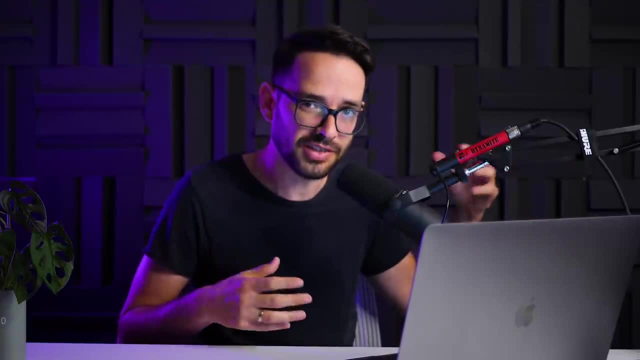 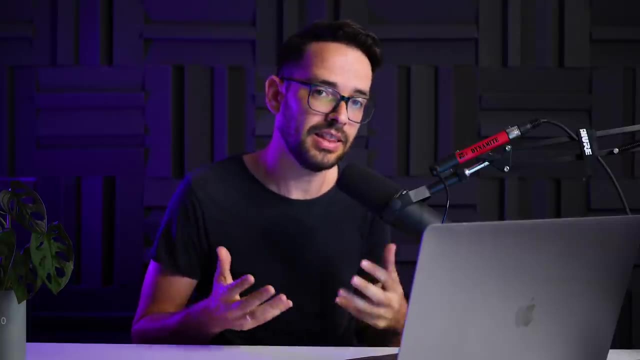 and white are actually colors, So people think about all the other colors that they have to be creative with, but actually black and white are not solid colors that you use. They also have their own meaning, So you need to take that into consideration. 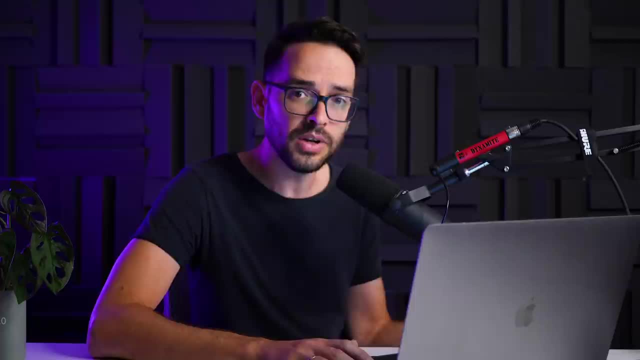 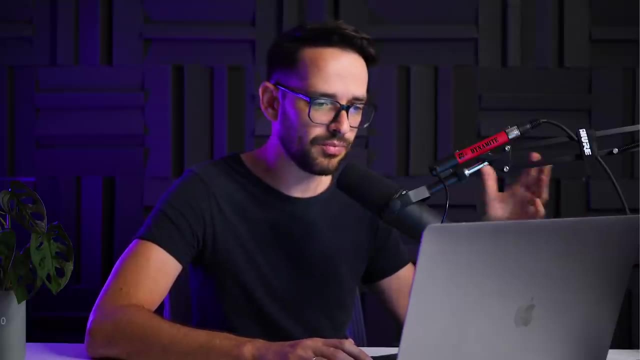 So that's the basic three color palette that we chose to. Now let's say: how are we actually going to use this? Now we're done with step two, Step three: how are you gonna apply that in your website? So the general rule that we talk about. 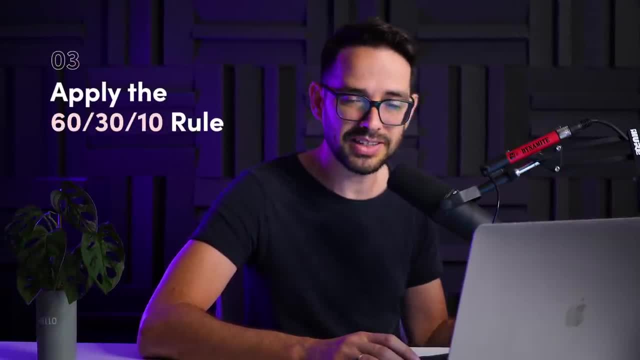 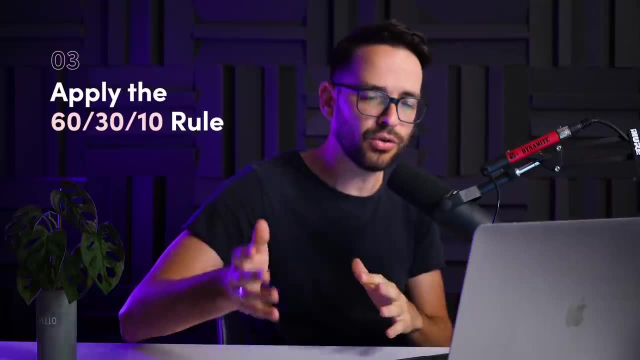 which is basically borrowed from interior design, is the 60-30-10 rule, And that's pretty easy to apply. You understand that the 60% is probably what's going to be your background And then 30% is going to be kind of main elements. 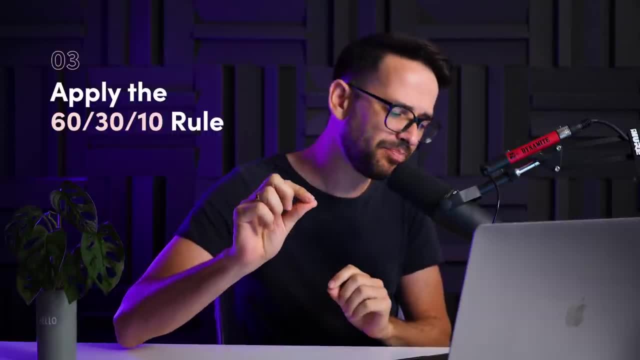 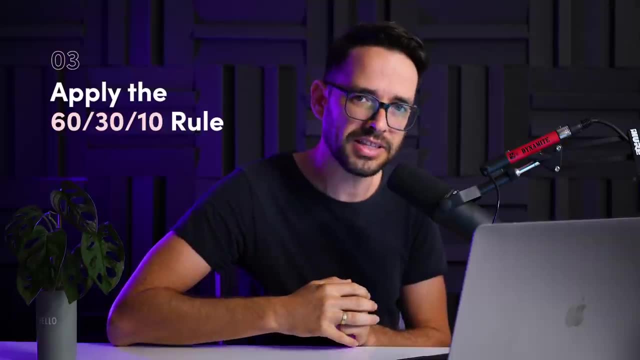 Sometimes those are texts or something like that, And the 10% it's what's called the ascent. It's just to give a little spark of color or something interesting to grab attention. Sometimes you'll use that for buttons: call to actions. 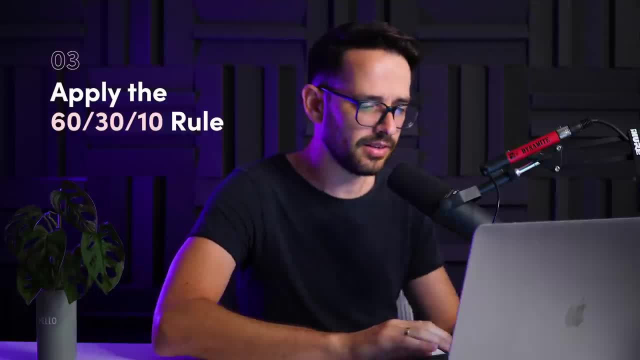 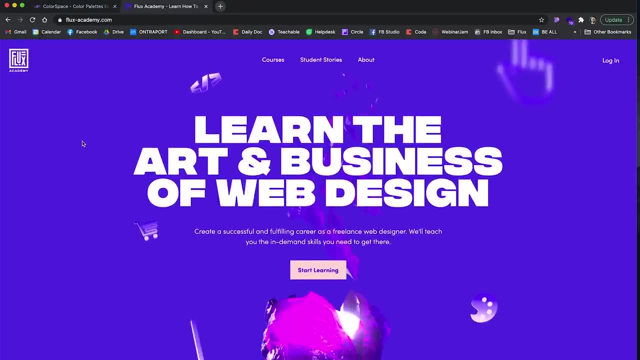 all of these kind of things. So let's take an example from Flux Academy and see how we've actually applied them. So here's the. let's go back to the top. So if you look here at the top, you can see that 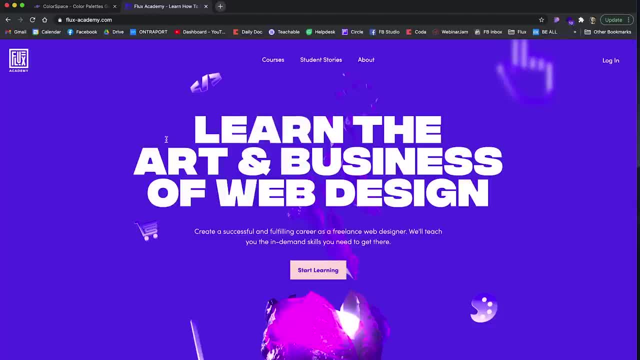 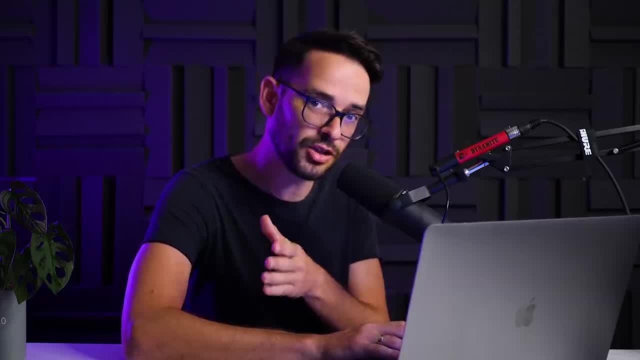 the 60% is actually the purple and the 30% is actually white. It's not black, because in this case black wouldn't be very readable on this color. So, as I've mentioned, for our palette, black and white are kind of interchangeable. 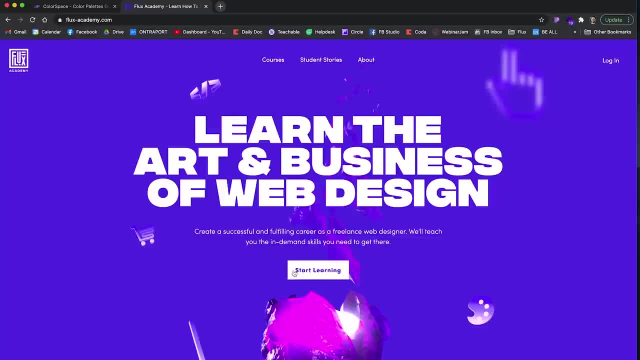 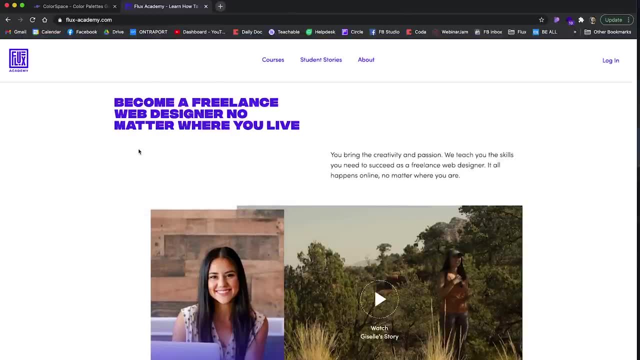 So here we use 30% with white and then we have the little purplish as an ascent, both for the button and for these other elements that we have here. However, when we scroll down, you can see that in these areas 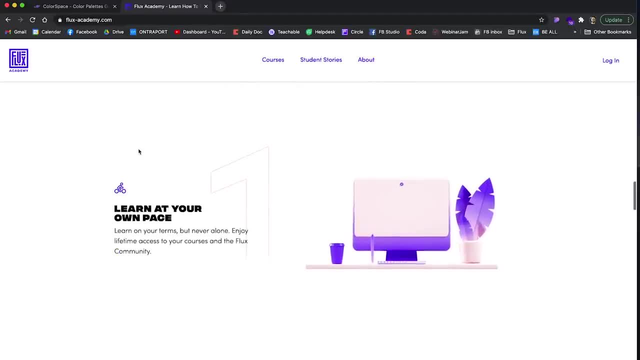 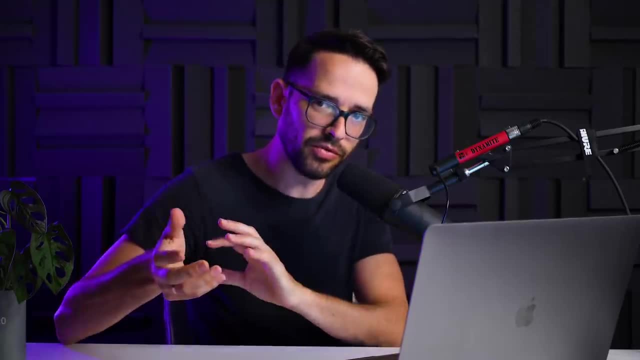 actually the palette has been switched out a little bit, So in these areas of the website the 60% is now the white right. It was kind of moved from positive to negative right, So now we have white as 60%. 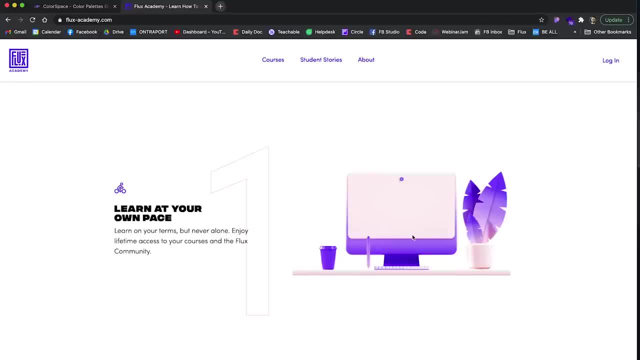 We have the actual purple, pinkish together as the 30% and then just a tiny bit of black, using the text here, And that's basically how we roll. So here's what I want you to take away from this. So you have, once you have, these three colors, right. 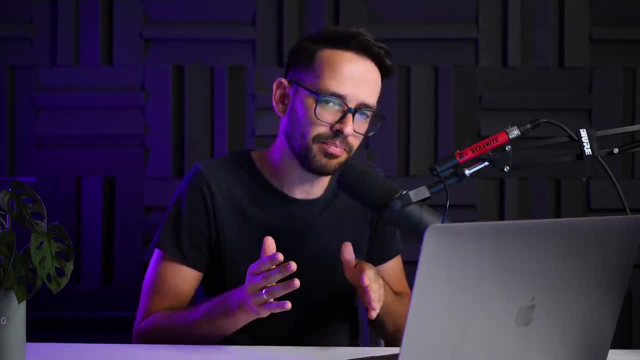 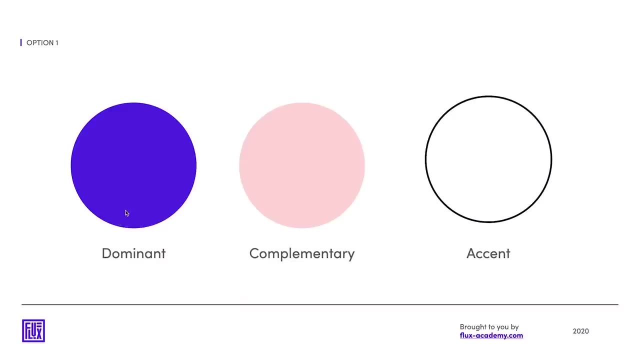 You can play around with them. It doesn't mean that they have to keep playing the same roles over again. So in this case, as I've mentioned, we had a part where the purple was dominate and white was the ascent, And then we had other parts. 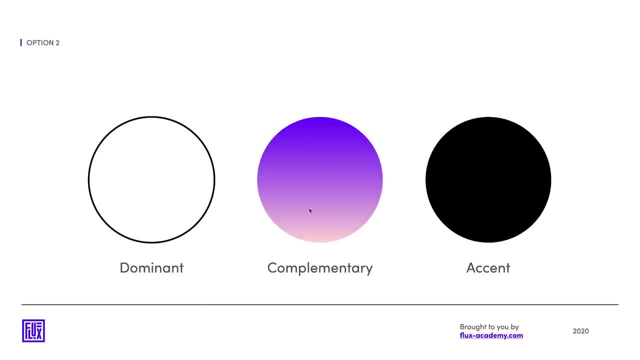 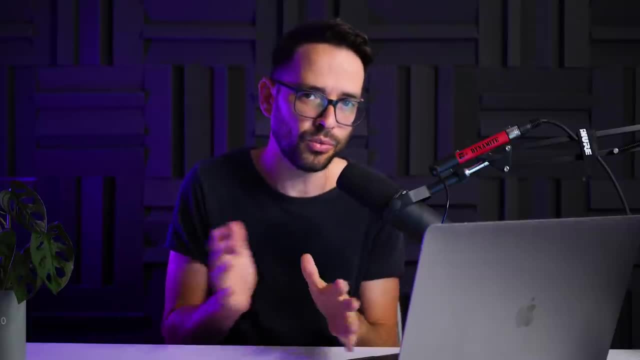 where the white was actually dominate, We've actually mixed the two colors into kind of a gradient or using both together as complimentary and the black was an ascent. So when you have a palette of three colors- and I still consider this three, even though we sometimes the palette is three with white- 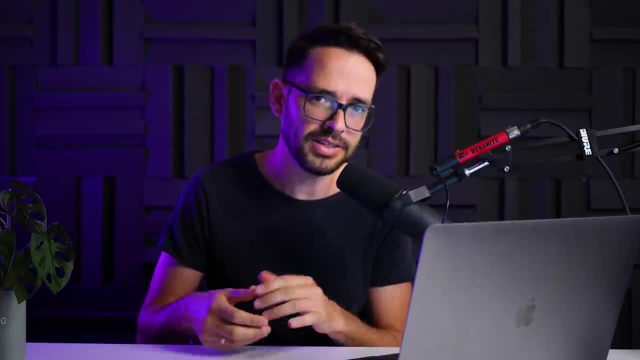 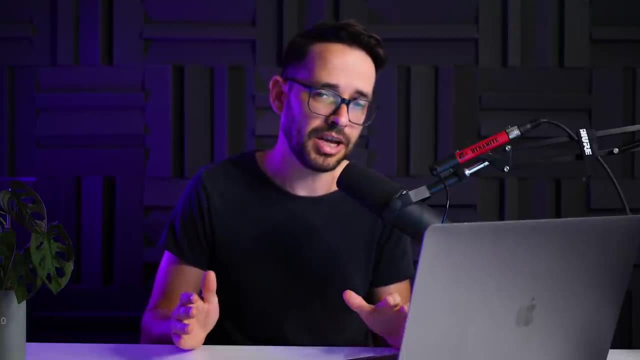 and three with black. you have a lot of different creative ways to mix them up using the 60,, 30, 10 rule, And that gives you a lot of versatility in your website. This is basically the process that I work through. 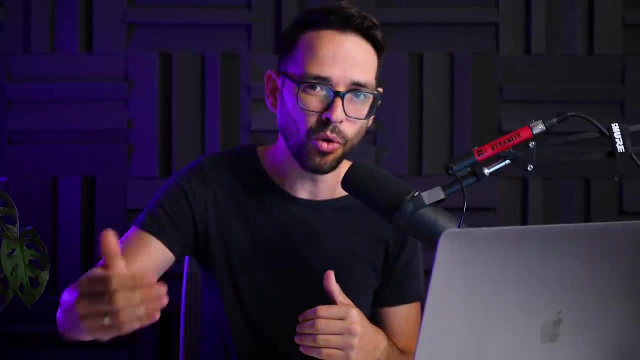 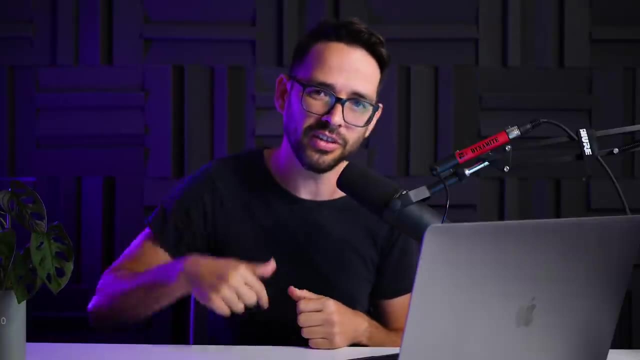 and that really simplifies my life. If you wanna learn more into how we apply this, how we use this with text, with images, with type, with strategy, you're welcome to check in below the link: our course, the 10K website process. and we'll see you on the next video. Bye-bye.